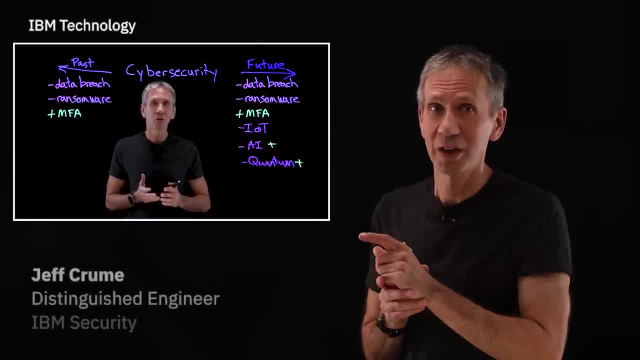 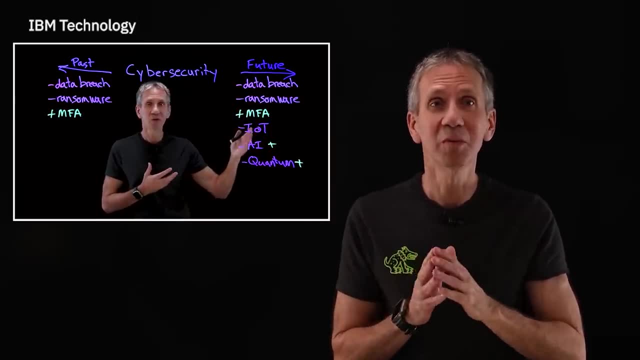 Last year I did a video on cybersecurity trends and in that I talked about artificial intelligence and I thought that was going to be important. It's turned out to be very important and it's going to be even more important as we go forward. 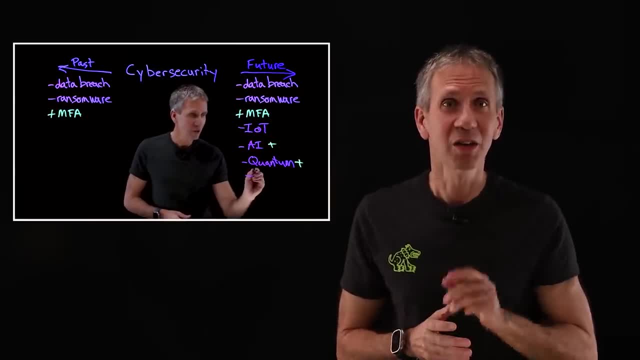 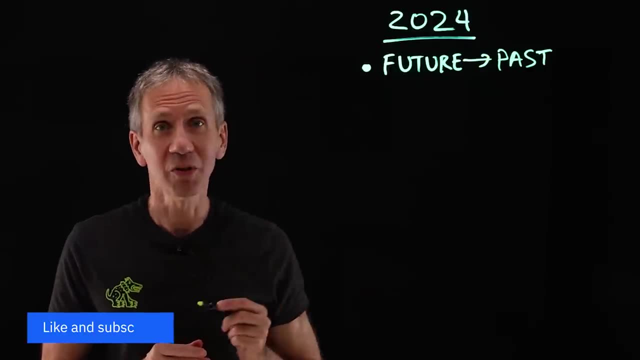 By the way, is my hair really that gray? In the next deepfake, we're going to fix that. Okay, let's take a look at the future. What I'm sure of is that the future will look something like the past, and, in fact, one of the things we'll see in the future are more AI-based threats. 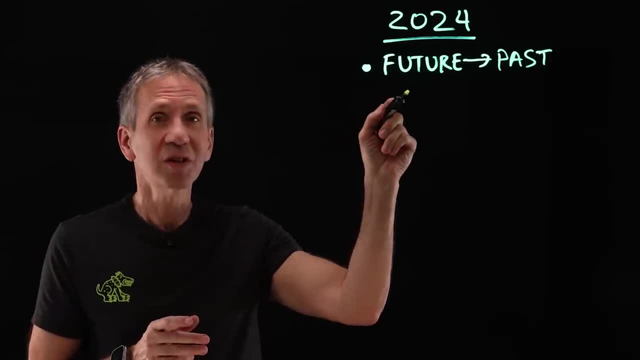 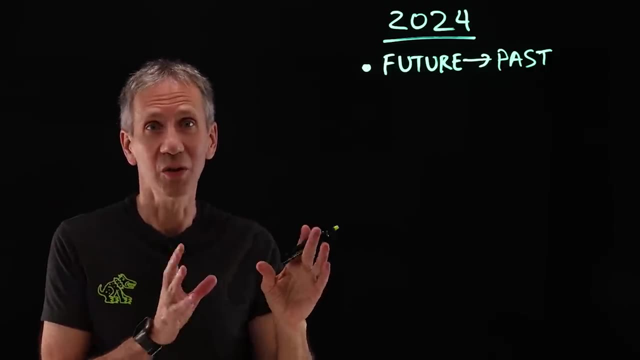 But more on that in a few minutes. What we're going to see, though, also is that change is the only constant, So that means things will be similar to the past, but there will also be new things that we're going to take a look at. 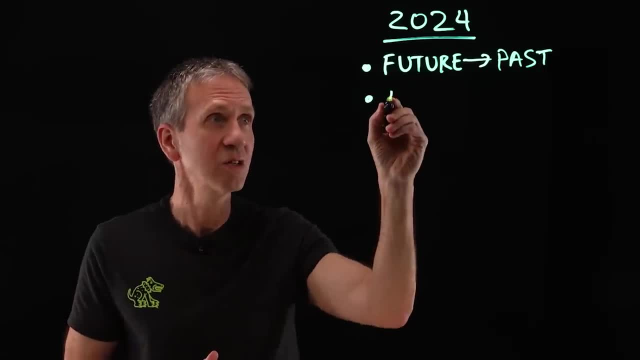 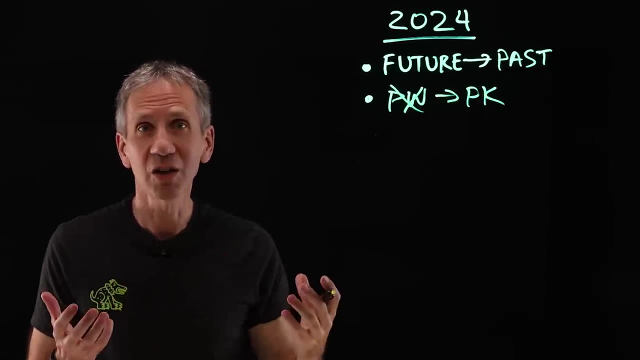 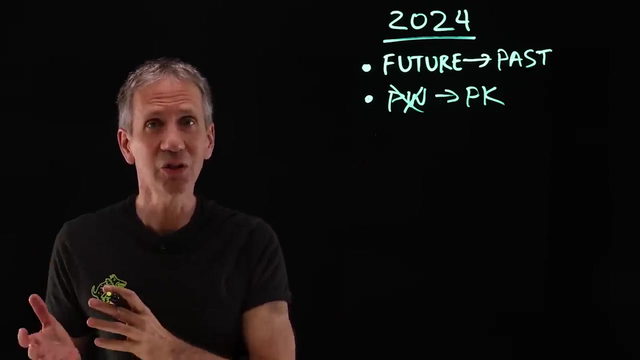 One of the new things that I think is on the positive side is that we're going to see a move away from passwords toward past keys. There's a new standard called FIDO that allows you to not have to send a password, but in fact do something that is simpler, easier to use. 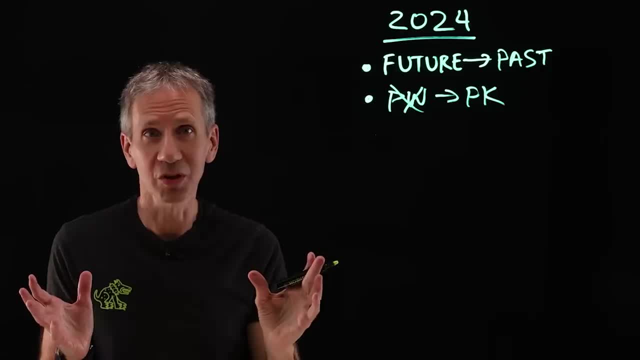 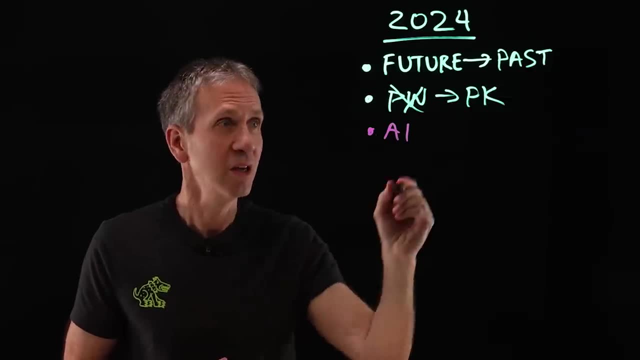 and more secure. We don't normally get to do both of those at the same time, and we're going to need it. And what's the reason for that? Well, because AI, as I mentioned, is going to be an increasing threat vector for us. 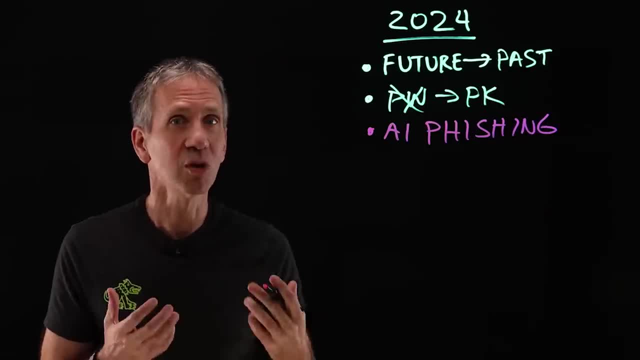 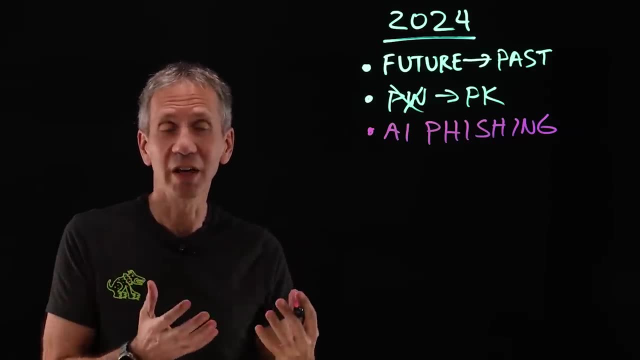 AI-based phishing emails are going to become more and more common, I expect, because they can generate what is very convincing emails to get people to try to log in or share their credentials in ways that they shouldn't, And this is a very efficient way. 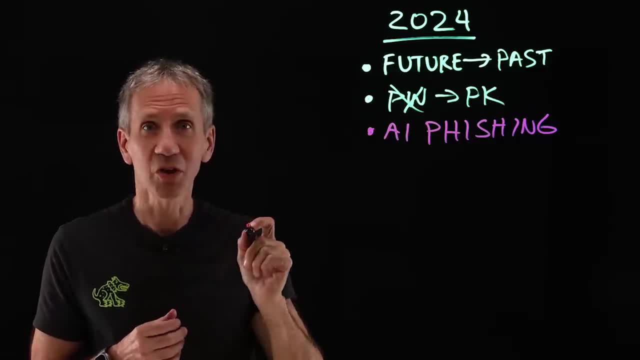 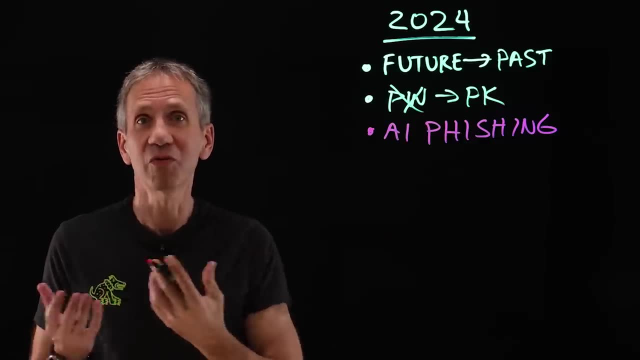 It's a very efficient way of doing it. However, if you don't have a password in the first place to send, if you only have something that is a secret that stays on your system, then there's no way for someone to phish that out of you. 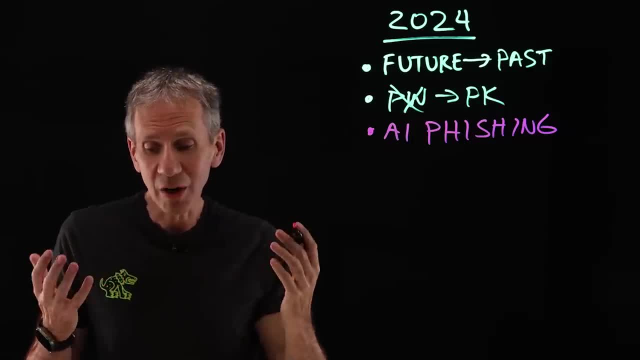 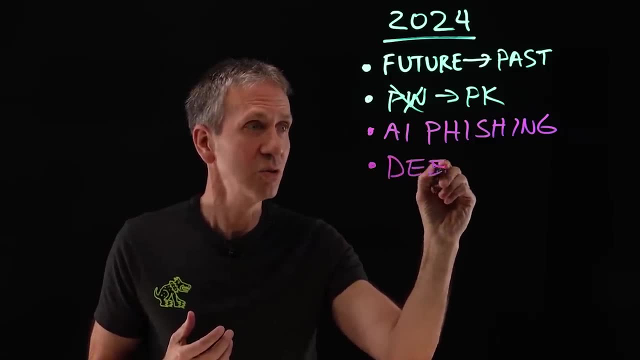 So this is going to be a good thing to try to help against that. Now there are other things that we can take a look at. that also in the AI space- generative AI- I think we're going to see an increased use of deepfakes. 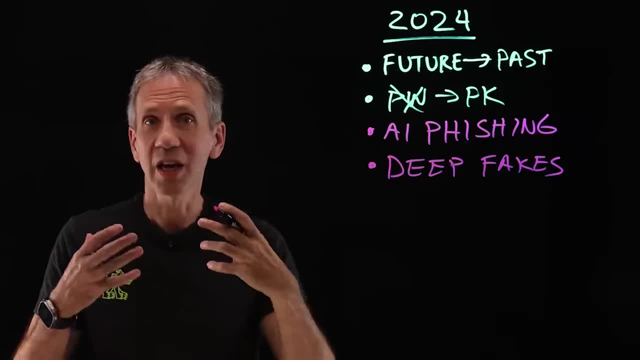 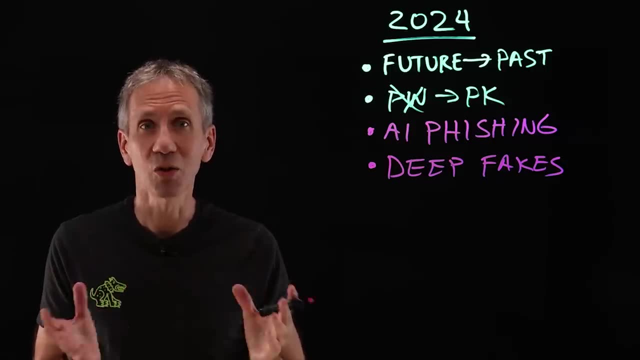 These are things where we simulate the voice, the image, the likeness of an individual And, in fact, deepfake technology has become so good and it is so prevalent. In fact, if you have a mobile phone, it's probably already built into your operating system. 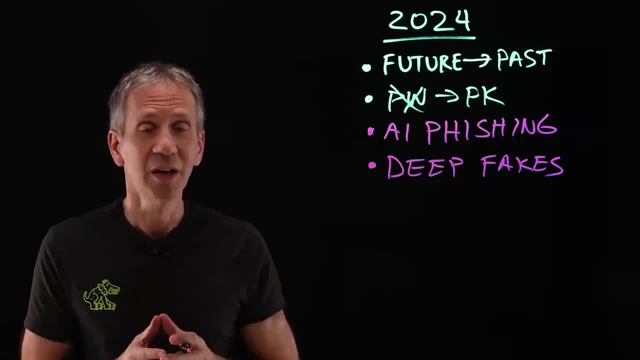 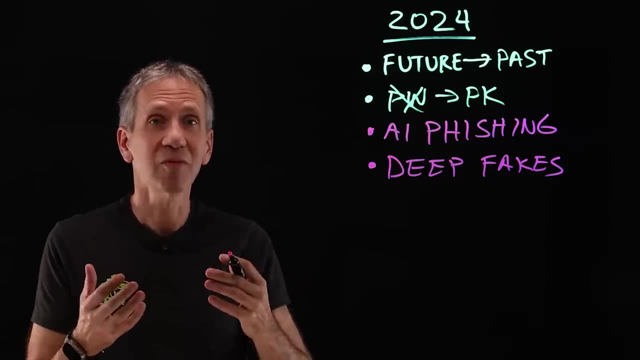 In most cases you may not know about it, but it's there. So you could use this kind of technology to fake someone out, have them believe something that's not true. For instance, have someone call a relative and say: I need money. 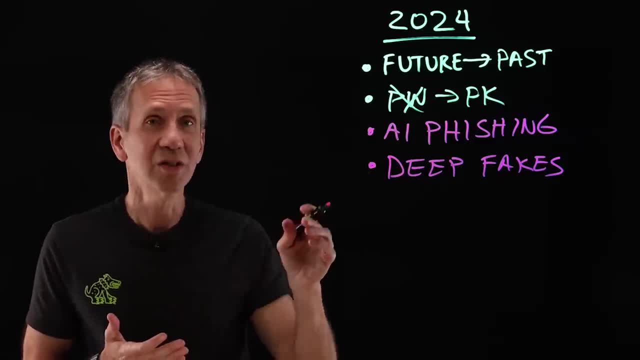 It sounds like it's your voice, So they send the money. So we're going to need to do more in terms of educating people about deepfakes and the threat in that space, because I think we're going to see more of it. 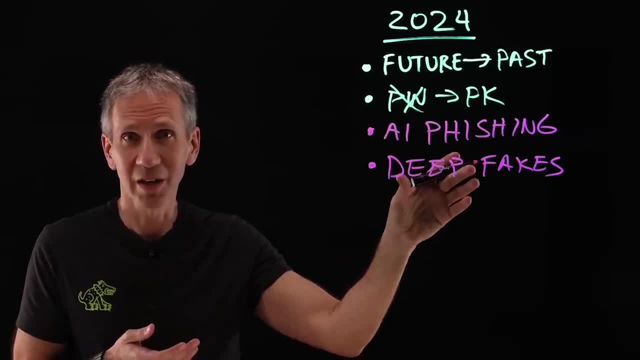 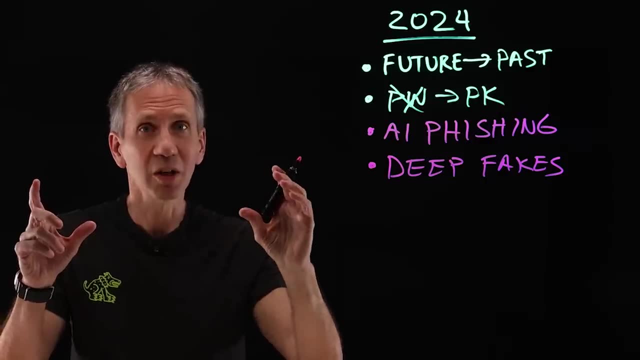 And, by the way, if you think deepfake detection is going to be a good way to go, I'm going to ask you to think again about that. Deepfake technology will always keep getting better and it will eventually be to the point where I don't think detection is going to work. 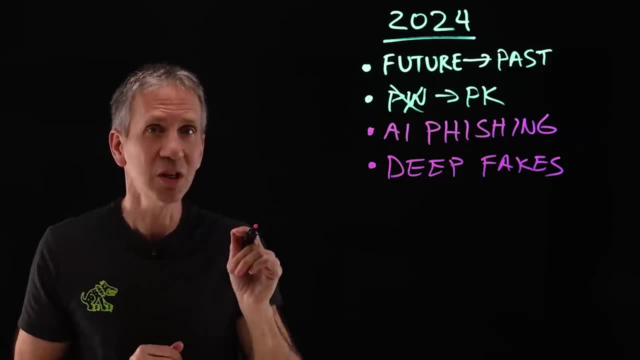 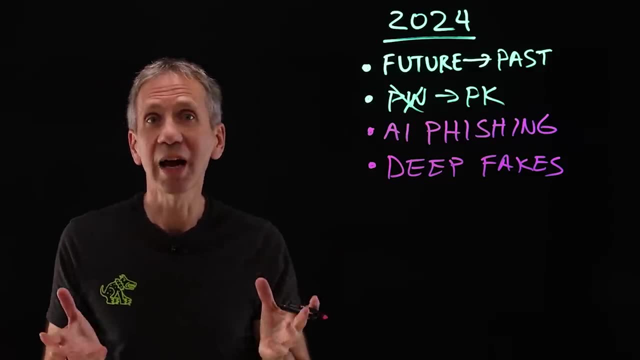 In many cases we've already seen this happen. So the focus needs to be not on detecting the deepfake with some sort of technology, but building security mechanisms around it, so that we're not reliant on the information that's in the deepfake itself. 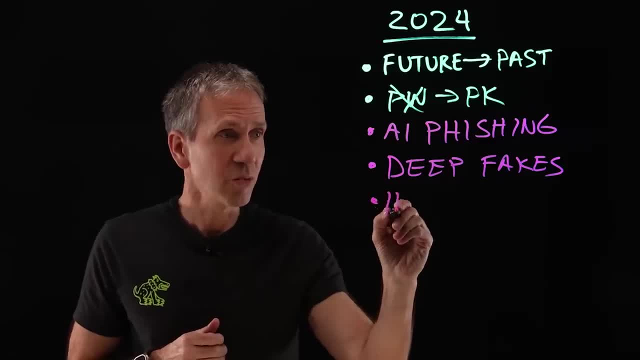 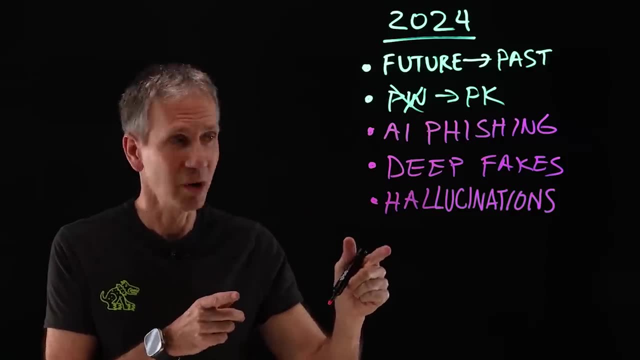 Other things that we're going to take a look at would be a threat that comes to us from generative AI, and that's hallucinations. And, by the way, you didn't think I was going to actually write that word out when I have a magic board that can autocomplete. 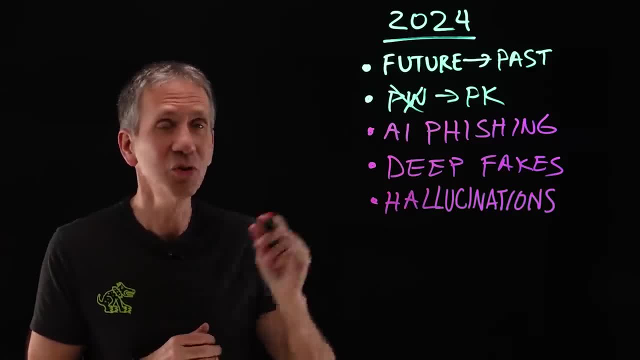 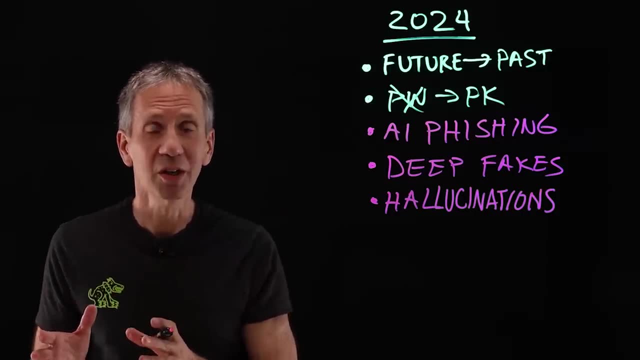 That's what generative AI does, right, So I'm leveraging that Hallucinations. We're going to be more and more dependent upon generative AI models and chat bots to give us information. The problem is, some of the information they give us isn't always right. 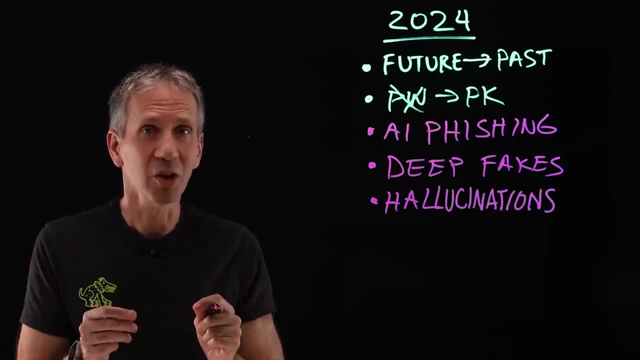 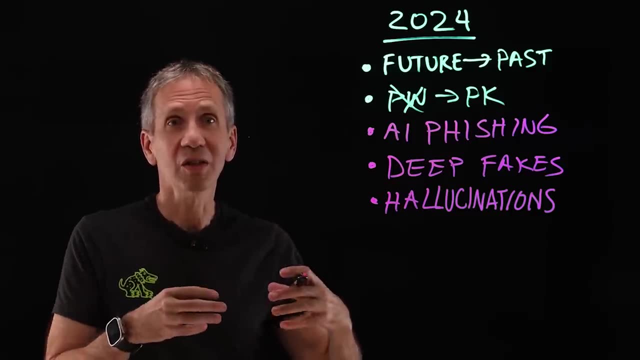 And we call those hallucinations And we're going to make decisions based upon that that could cause security threats to us. So my hope is that there will be other technologies- things like retrieval, augmented generation or what we call RAG technology- that will help. 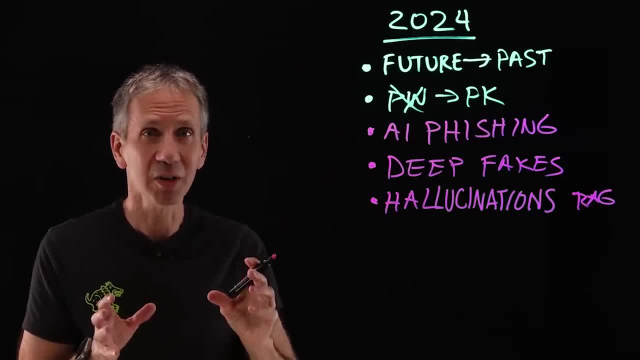 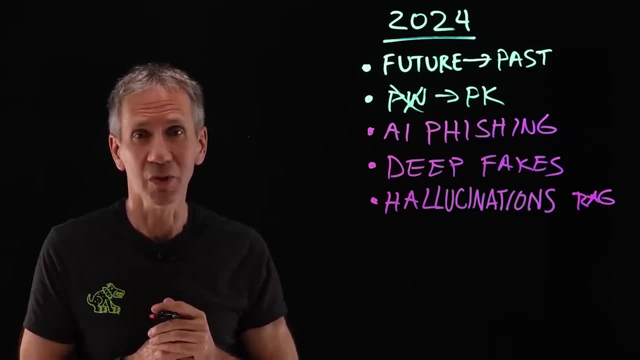 reinforce and make this system better and more accurate. Other things that we can do to tune the models and train them better so that they don't hallucinate nearly as much going forward. And then, finally, I'm going to say something. I want to leave you with a 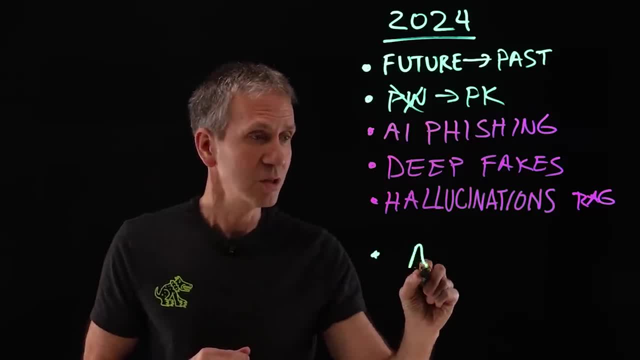 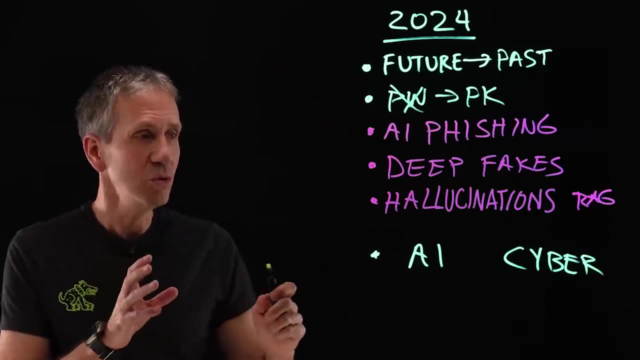 positive in terms of a look at the future, And that is there's this symbiotic relationship between AI and cybersecurity, And that is we're going to use AI to do better job of cybersecurity. In fact, there's a lot of things that we 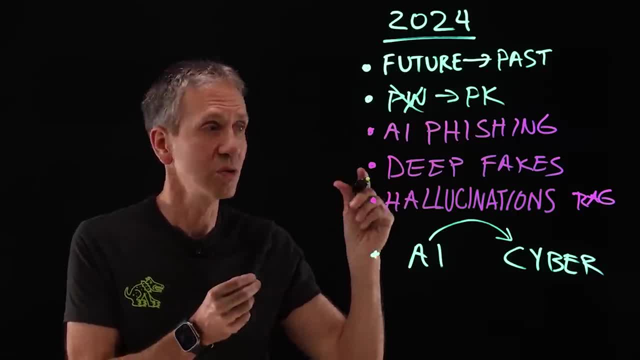 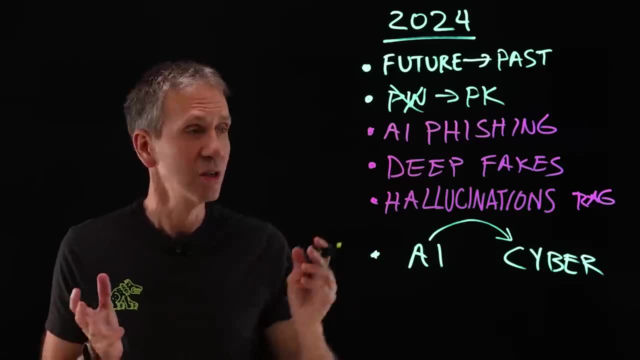 can do in this space to leverage generative AI in order to better think about the way someone would attack us, Also summarize cases and things of that sort. So I think we're going to be able to do a better job with cybersecurity by leveraging AI. 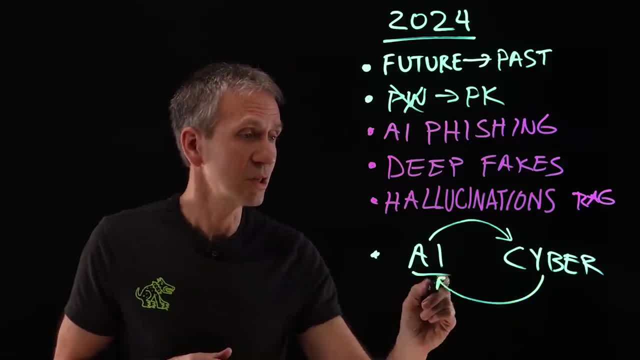 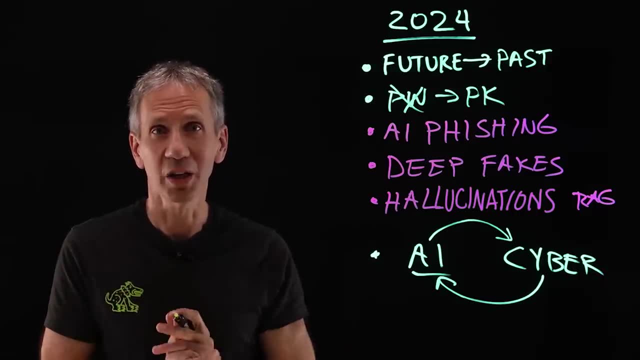 By the same token, we're going to need to use our cybersecurity skills in order to secure this AI, so that it can be trustworthy, so that we can in fact believe that the information it gives us is true. OK, that's the future. 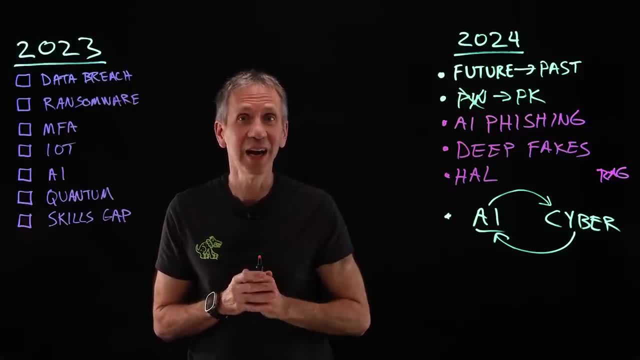 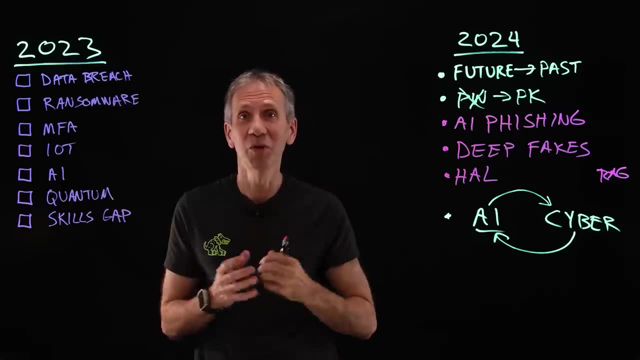 And it's not a big surprise that the future is very AI heavy. However, there's a lot of existing threats that have continued to persist and will continue to persist as we move into the future. Let's take a quick look at the scorecard from last year's predictions and see which. 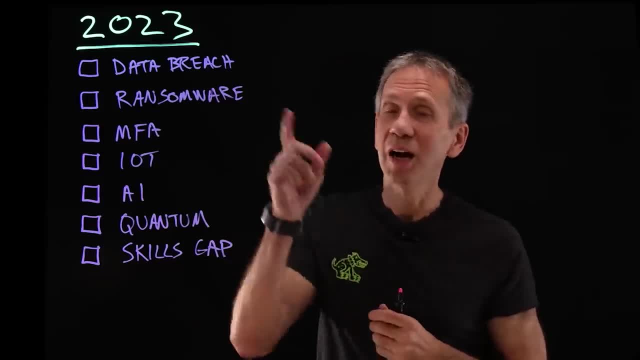 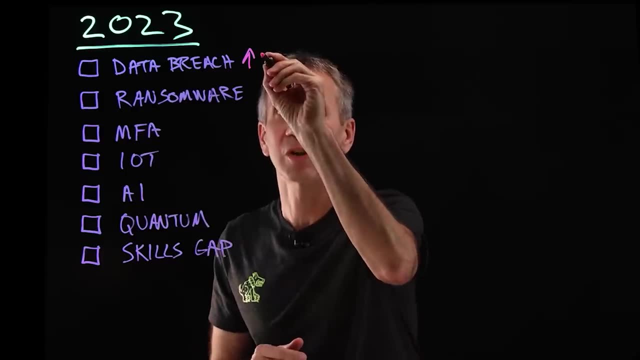 ones of those actually came true and which ones carry forward. I mentioned data breach last year when I did the video, And in fact it turns out that the cost of a data breach has continued to increase. In fact, now we're on the order of four and a half million dollars on average. 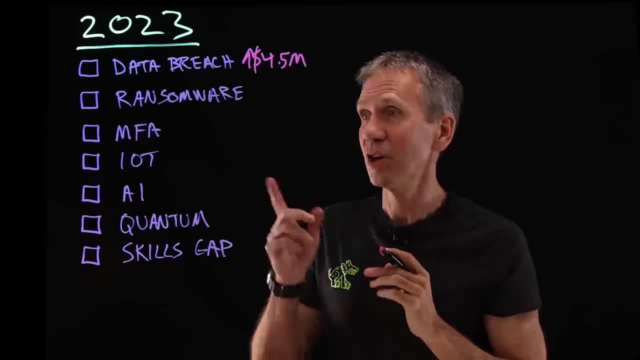 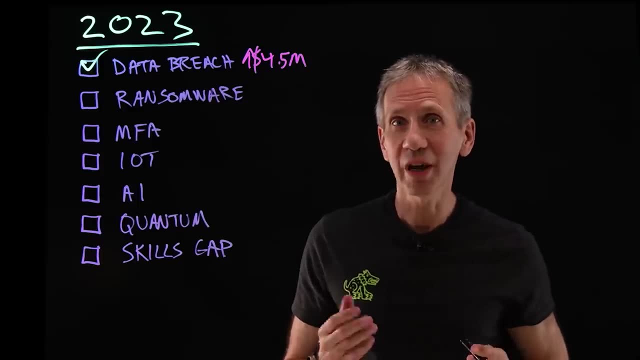 worldwide and in the US that number is almost twice as high. So that one I'm going to say: yeah, came true. Ransomware- in fact we've continued to see ransomware persist. The overall numbers are a little bit down. 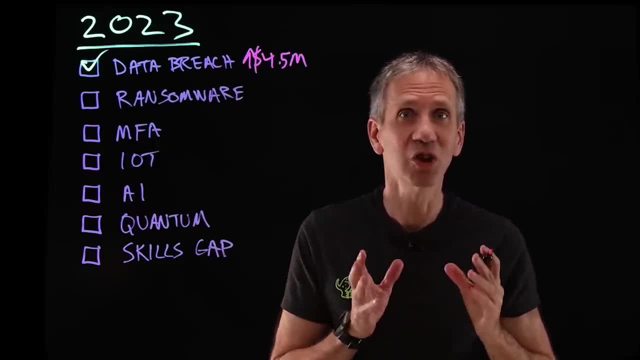 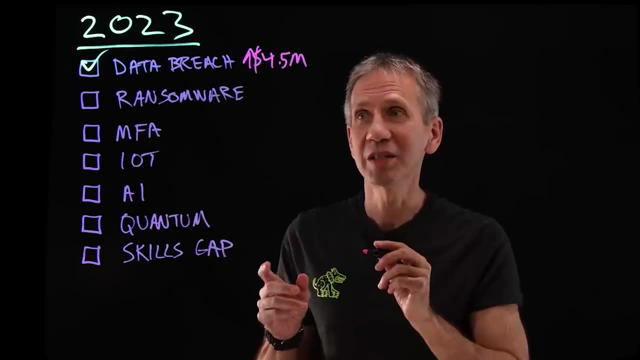 but the amount of time it takes to run one of these attacks has changed dramatically. This according to the X-Force Threat Intelligence Index, which says that back in 2019, we were looking at 60 days on average to deploy one of these. 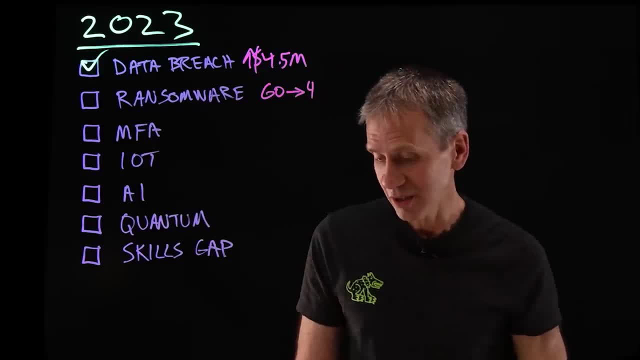 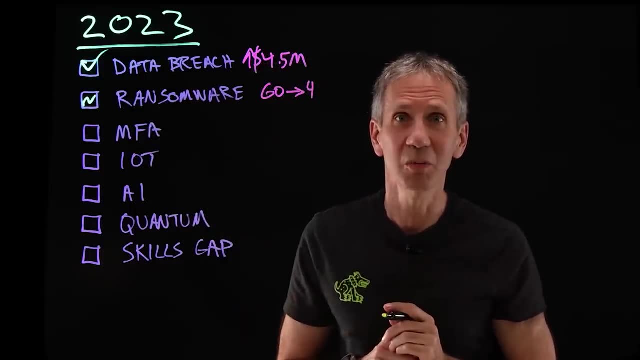 Now we're down to about four days. So this is kind of a mixed bag. You know this is it's sort of true, sort of not true. But ransomware is going to continue to be a threat, and it's a faster threat than it used to be. 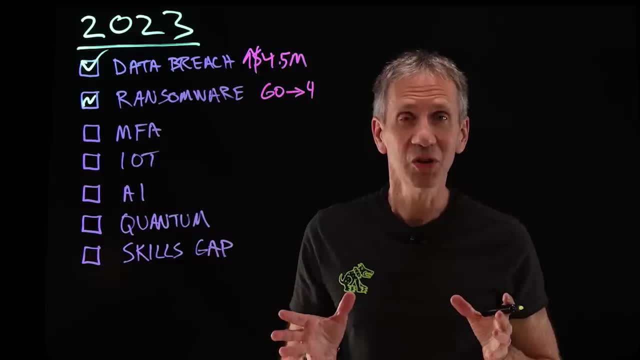 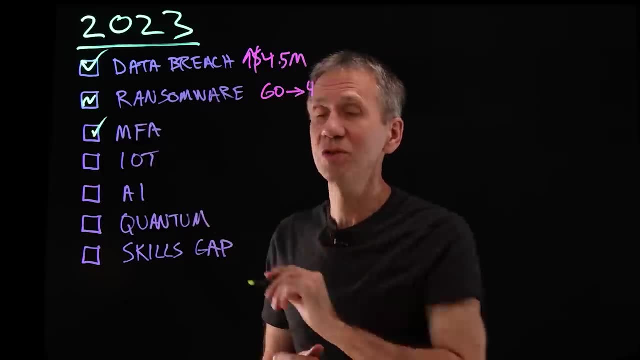 Multi-factor authentication. I don't know about you, but I'm definitely seeing more websites that are offering this as an alternative, And I'm taking advantage, and you should as well. I think we'll continue to see a lot more of that as we go forward. 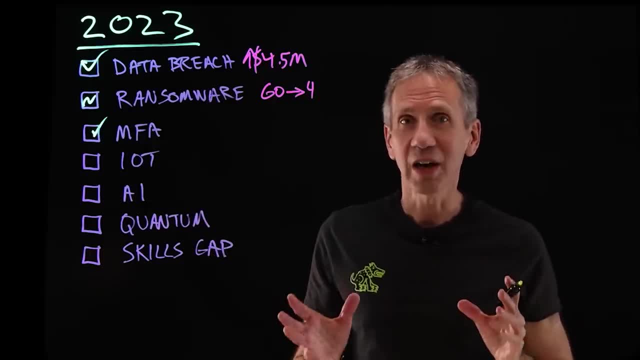 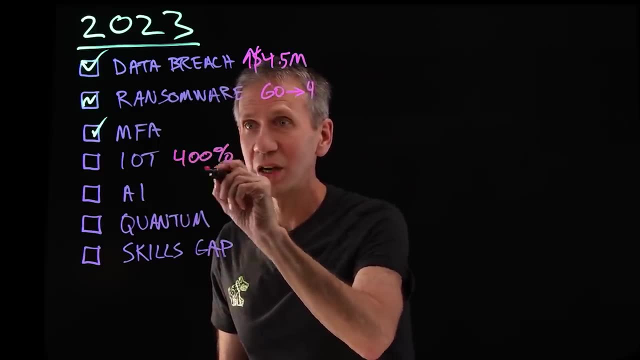 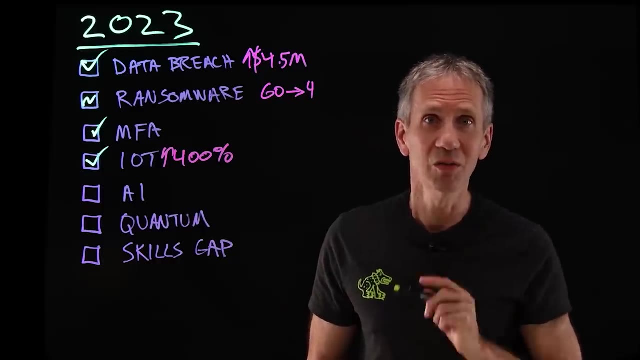 IoT- Internet of Things- threats. Yes, In fact we've seen there was one study that came out that said there was, in fact, a 400 percent increase in IoT attacks in this year, 2023.. So that one is definitely continued.